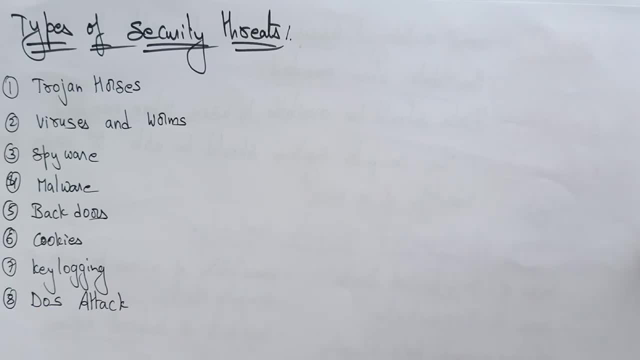 going to explain all these different types of thread. i want to give a a little bit uh information regarding the security threat- actually a computer uh security, or whatever i explain, or the it security, if you talk about your personal computer security or if you talk about the it. 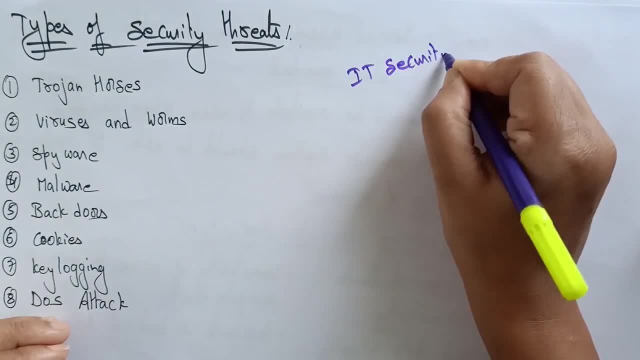 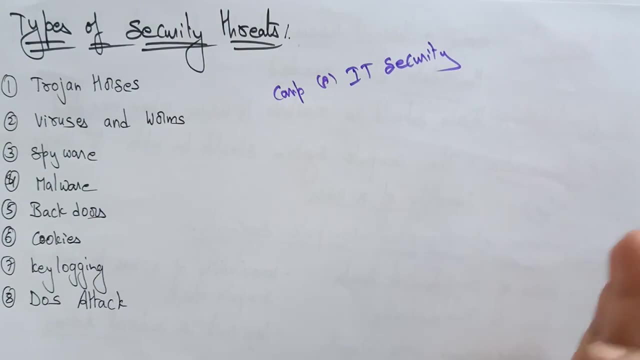 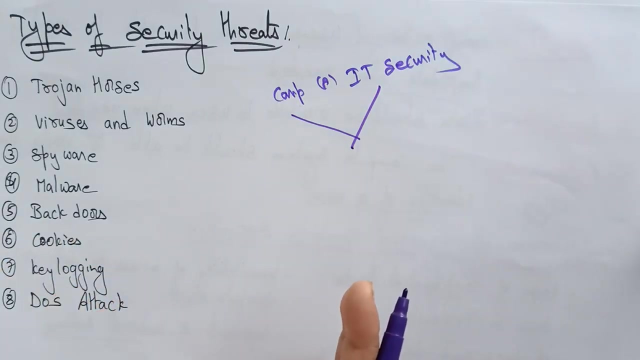 it security. so either your personal computer, okay, or it security, which is a global demand. so everything- the computer security or your personal or it security, everything is a global demand to protect out computer system from malicious attackers from doing any damage to your hardware, software and your computer security. so this is a global security threat. so if you talk 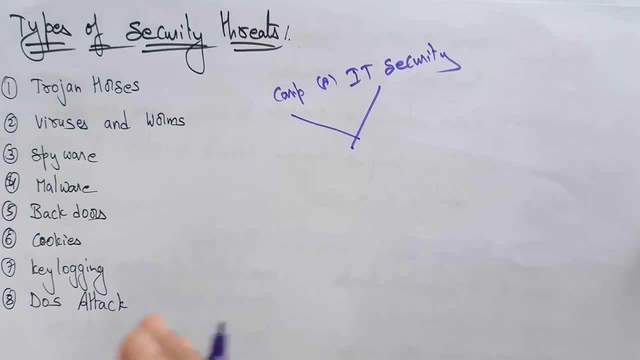 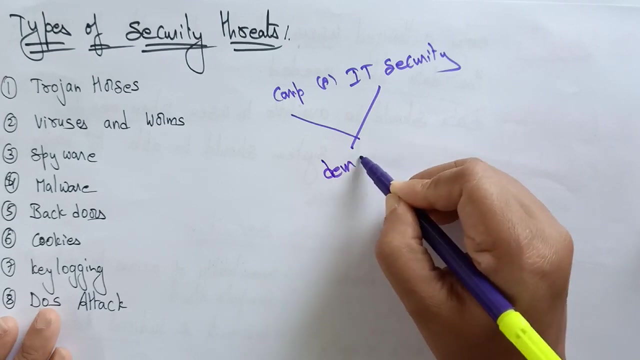 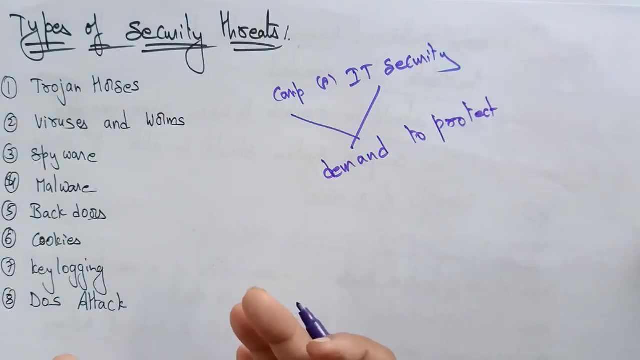 about it as well as the disruption of services provided. so that is a main global demand. nowadays everyone is focusing on that, not only uh the it organization, the personal computer systems or whatever the uh different organizations. everyone is demand on the protection demand to protect. to protect what? to protect out the computer systems from malicious attackers. so many it hackers will. 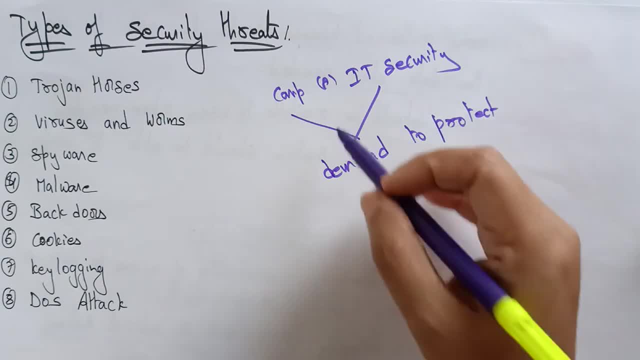 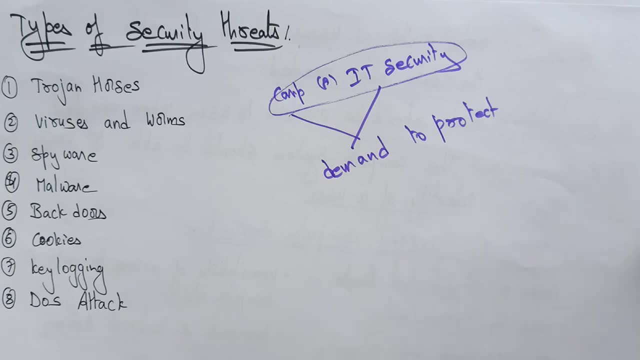 be there so to protect our computer systems from malicious attackers. so many it hackers will be there so to protect our data. all these it securities and organizations are concentrating on these security threats. okay, so which are going to damage our hardware? it is going to damage our hardware software. 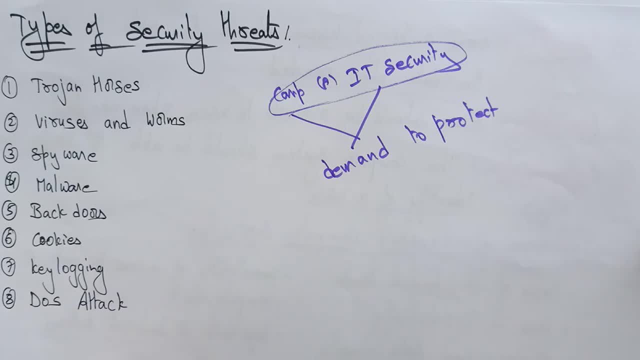 and even also some disruptions will be occurring on the service provided. so the computer security involves controlling our physical access as well as protecting against the harms that occurs. okay, so it is what it is going to do, mainly what is going it is going to do. it is going to what? uh, controlling and physical access. so, whatever the physical access you are, 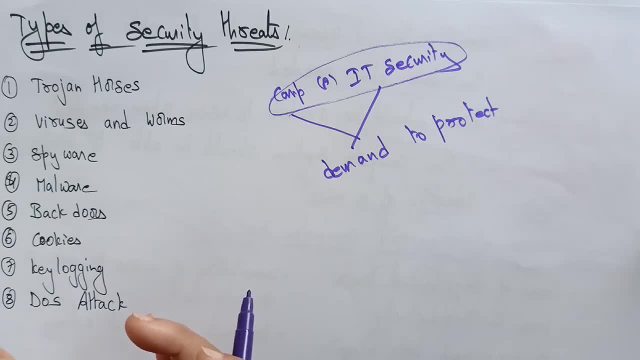 doing so, it is keeping some concentration on the physical access as well as the protection against the harm. suppose any of these attacks are coming. it is going to work on against these harms. so the how these uh threats will occur, how these threats will occur. these threats will occur via network. 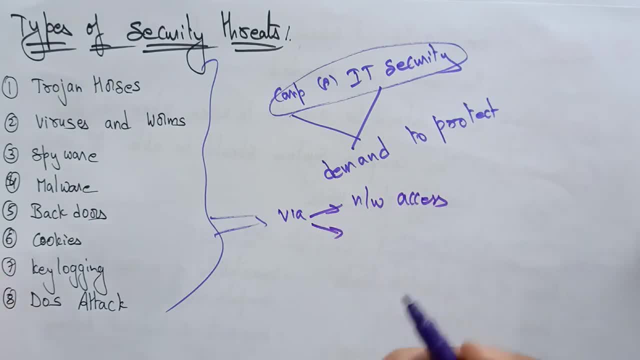 access obviously means: uh, these attacks, the security threat attacks, will be a occur via the network access or a data access. data access means, suppose, while you are working on these uh pen drives or something like the email attachments, the data access or even the code injection. also suppose, if you want to, some uh. 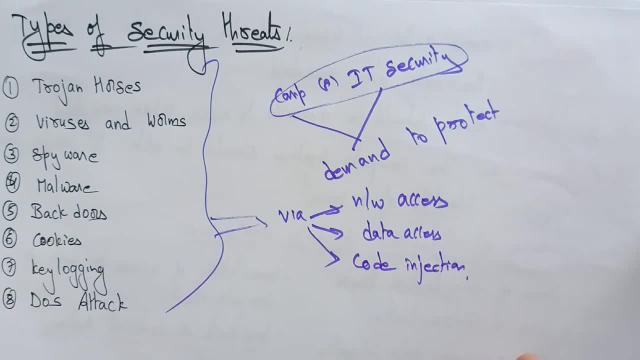 install some softwares. okay, so in that softwares- uh, a malicious code that is, which is going to harm your system. that is going to affect your system. it is going to be more dangerous than ever, but basically this procedure is based on pure tanto that is going to be installed in your system and it it attacks your uh system as well as it steal. 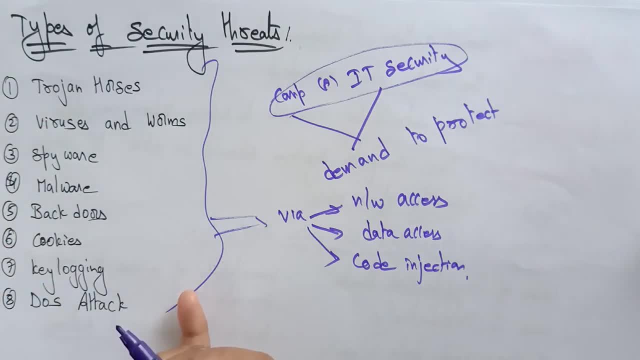 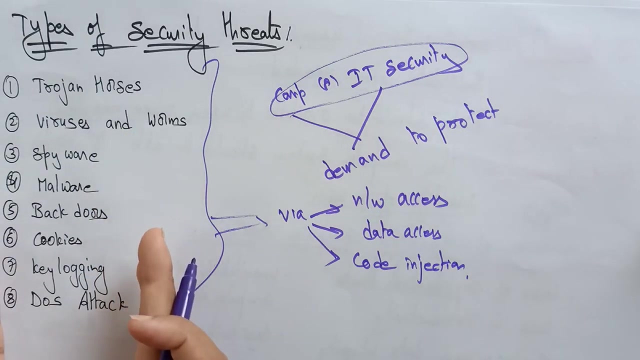 your data, and some, some- uh some- security threats will be concentrating on stealing of data, and some security threats will be concentrating on damage your hardware or software, or some will be disruption of service provider. like that, each security threat will doing some different works. so these all these- 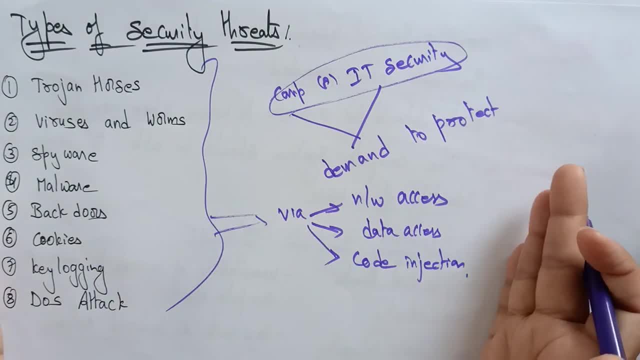 attacks will be coming via network access or via data access or via from the code injection. so what the attack attackers often think let's, let's have discuss about it. the attackers. whatever the attackers are there, the attackers often think a head than a problem solver. suppose you're the. 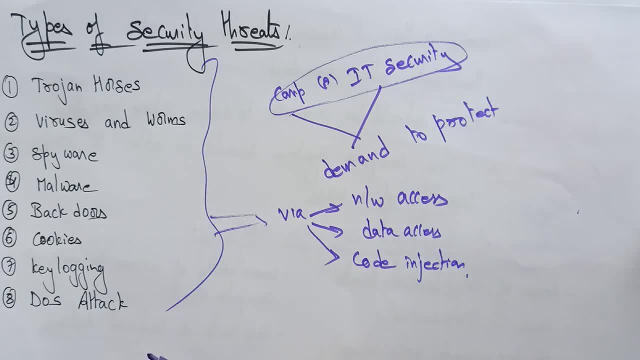 problem solver. you want to uh maintain some uh security, uh avoid the security threats, so you want to create a software which is going to protect your system. so obviously, the attackers who are created these type of attacks are the ones who are going to protect your system. so obviously, 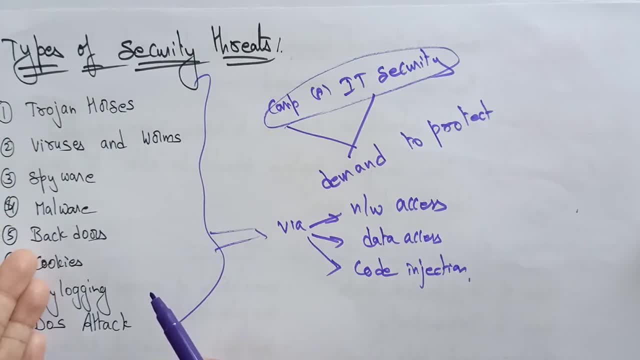 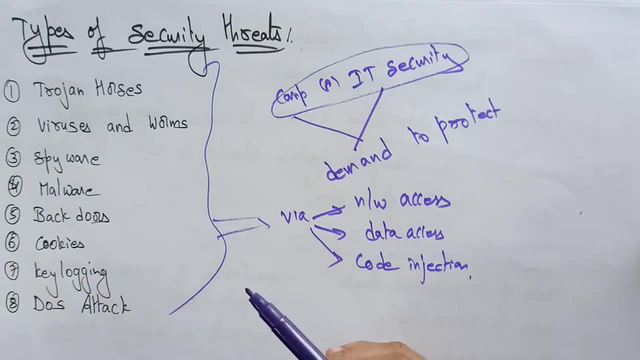 codes: okay, which is a malicious codes. the malware functions: okay, the the malware code. so these attackers often think ahead than a problem solver. so always keep in mind that they are frequently trying or using the different attacking techniques and methods. okay, suppose you have to think like that. what you have to think, suppose, if you are creating any software which is going to protect. 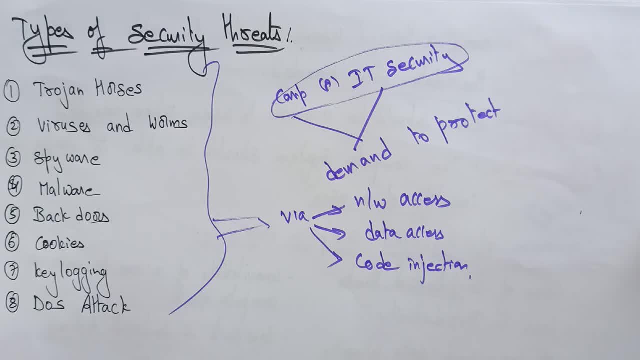 your data. you have to think ahead than the attackers like you have to frequently trying or using the different attacking techniques. so what are the different attacking techniques that are created? so you have to concentrate on that and you have to think about the methods that we can be override that. so the there are several types of computer security type threats in modern